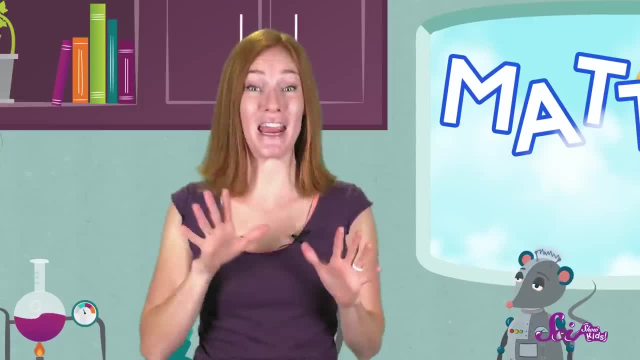 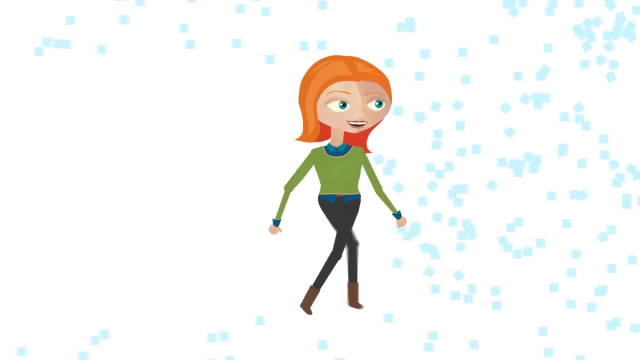 That's what scientists call just stuff. Everything is made of matter: The parachute, the air, the ocean, you, me, everything. And since air is made up of matter, when you walk through the air you're actually pushing matter out of the way with every move you make. 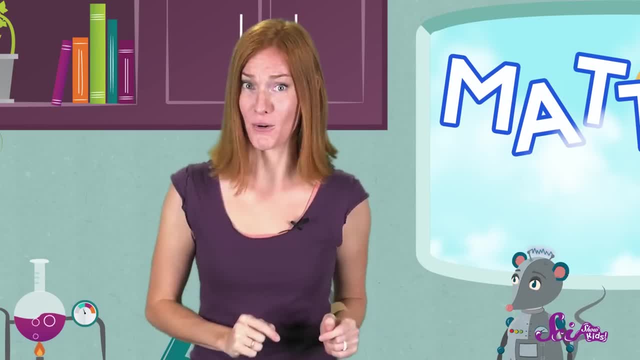 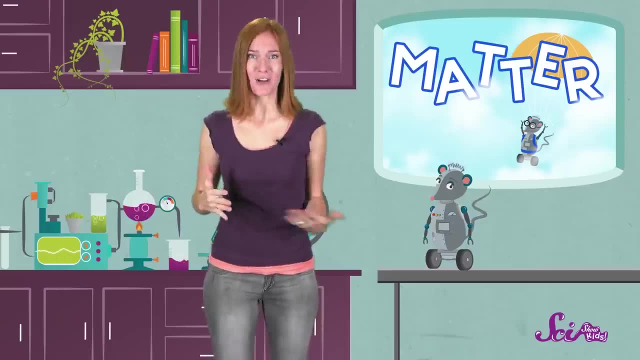 But here's the thing that matter is pushing back on you too. You probably don't feel it when you're just walking around, but when you start running, you might feel it a little bit. And when you start to go even faster, like when you're speeding around on your bike, 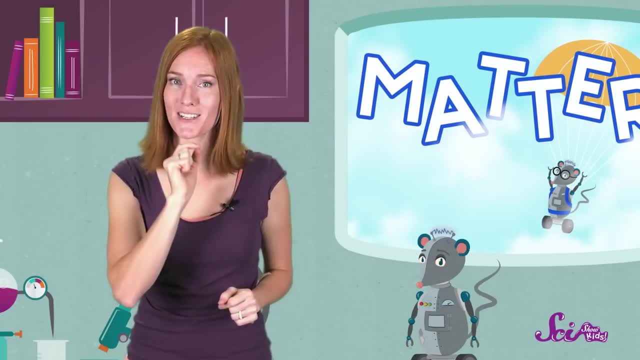 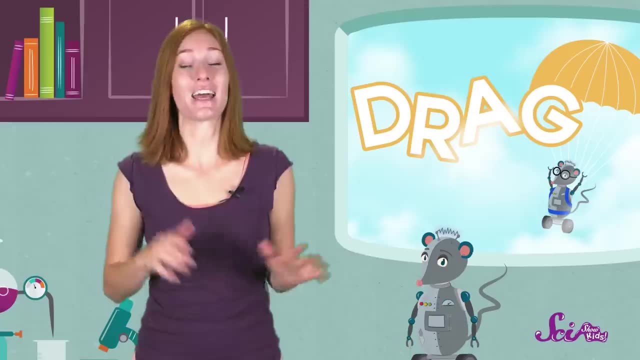 whoa. That feeling is the air pushing against you. And this force has a name: It's called drag. Drag is the force of the air pushing back on you or on anything when it moves, And the faster something is moving, the more drag it feels. So you don't really feel the force of the air as you walk around. But have you ever held your hand outside the window of a moving car? That's some serious drag. You can feel the air pushing against your hand and it can be hard to even keep it still. 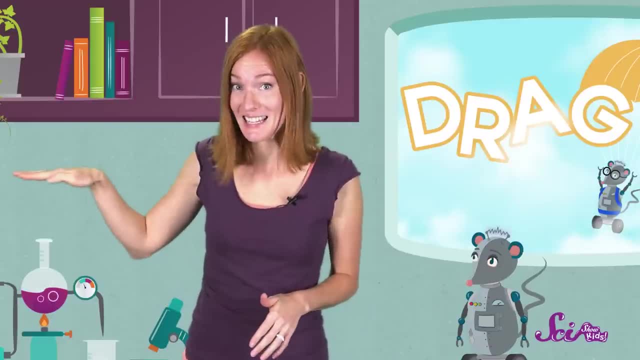 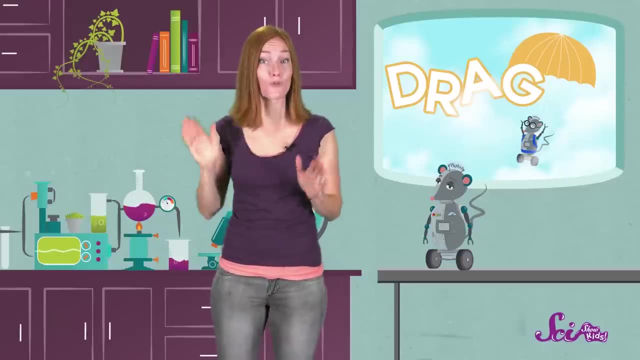 But have you noticed that it's easier to hold your hand flat like this than it is to hold your hand, so your thumbs point up? Why do you think that might be? It's because when you hold your hand straight up like this, more air is bumping into your 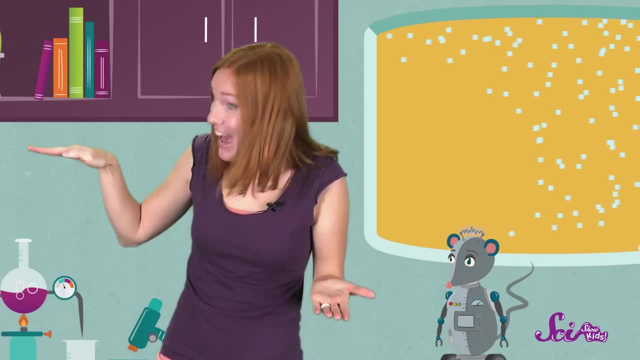 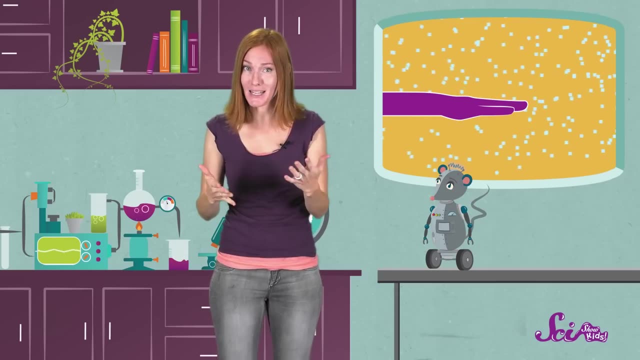 hand. That means more drag. But when you put your hand flat like this, only a small part of your hand is pushing the air out of the way. There's less of your hand for the air to run up against, which means less drag. so 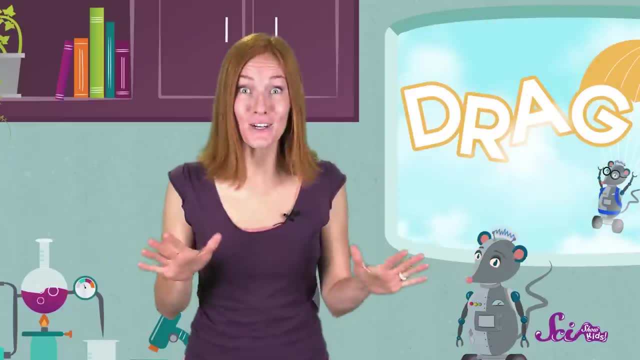 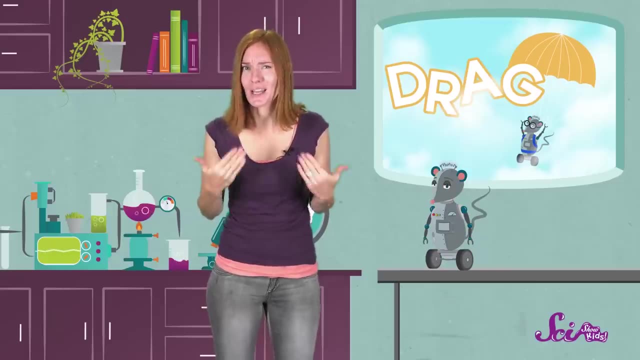 your hand can glide through the air more smoothly. So what if you're a skydiver and you're jumping out of an airplane? How do you slow yourself down so you can land safely? You'd want to do something that would make more air bump into you. And that's how a parachute helps. It makes more space for the air to run into, so it creates more drag. There's so much drag on the parachute, so much air pushing against it, that it slows down your fall so you can land safely. 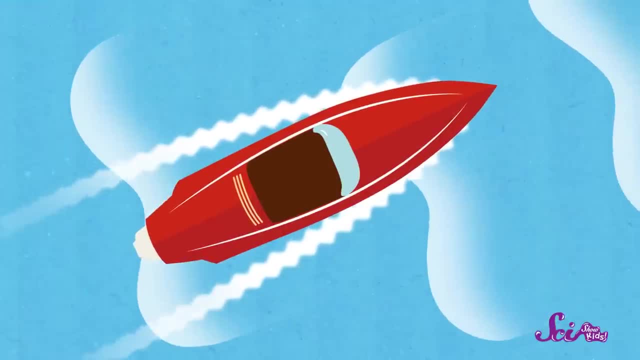 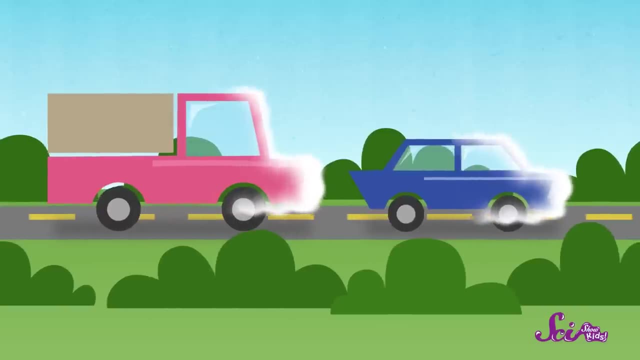 Now a lot of other things experience drag too. When a boat moves through the ocean, the water that pushes back against it is also making drag, And cars and trucks experience drag when they're driving down a highway. A little car feels less drag than a big truck because it has less space for the air to. 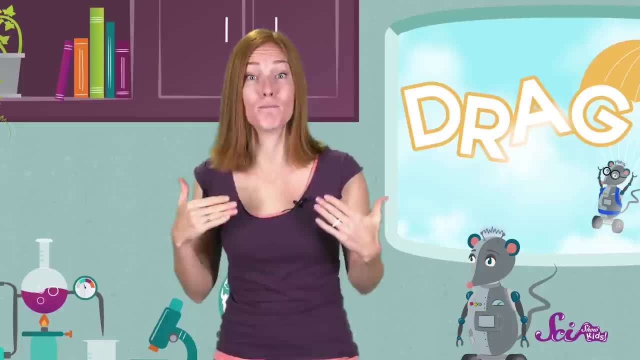 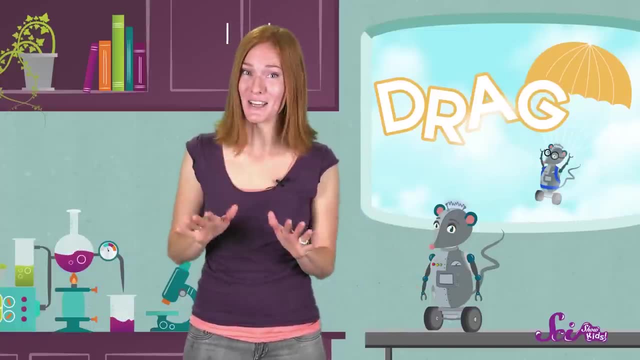 push against it. So drag is the force that you feel when you're moving through something like the air And that something pushes back. It may slow you down, but it's what makes lots of things, from skydiving to playtime with parachutes- possible. 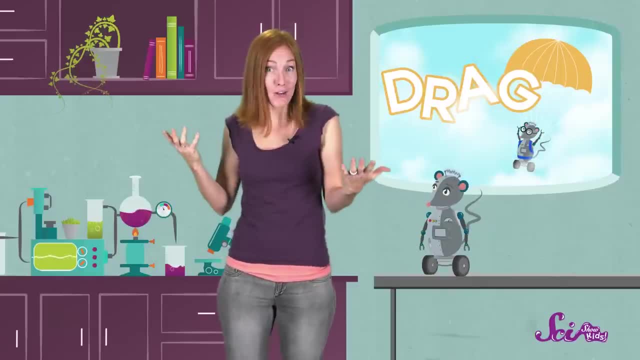 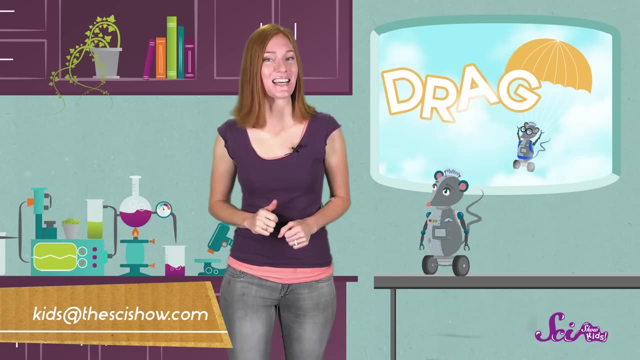 Thanks for joining us on SciShow Kids. Do you have a question about parachutes force or anything else at all? Ask a grown-up for help and leave us a comment down below or send us an email to kids at thescishowcom. And we'll see you next time.